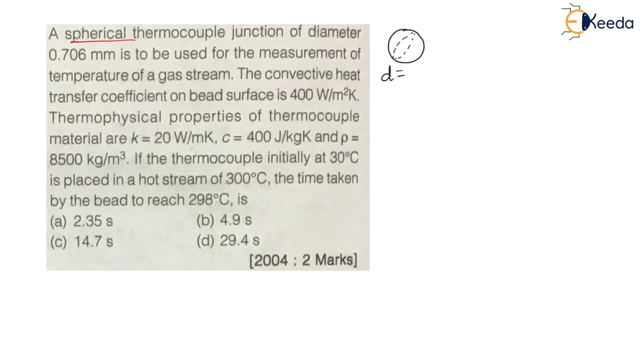 junction of diameter: 0.706 mm. Here diameter is given 0.706 mm, which is nothing, but diameter is equal to 0.706 into 10, to the power of minus 3 meter in terms of meter. Now here a spherical. 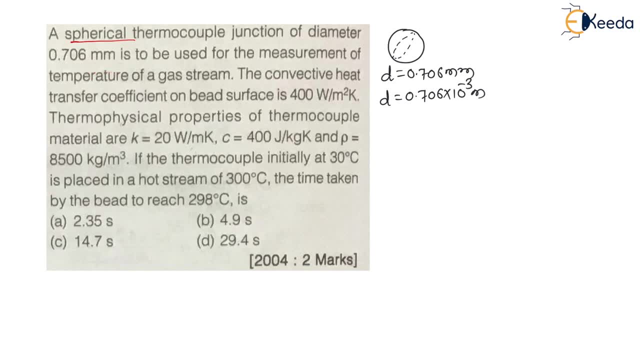 thermocouple junction of diameter 0.706 mm is to be used for the measurement of temperature of gas stream. The convective heat transfer coefficient on the bead surface is 400 Watt per meter square Kelvin. Therefore, here they have provided value of pH which is nothing but 400 Watt per meter. 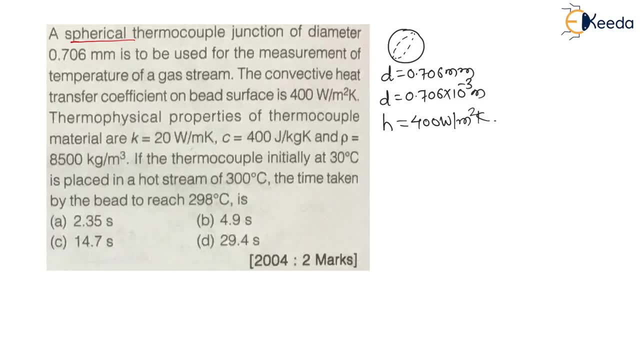 square Kelvin. Convective heat transfer coefficient is H. Thermophysical properties of thermocouple material are: Thermal conductivity is given. Thermal conductivity is given. Thermal conductivity is given. Specific heat is given and density is given. Let us write them. Therefore. thermal conductivity is: 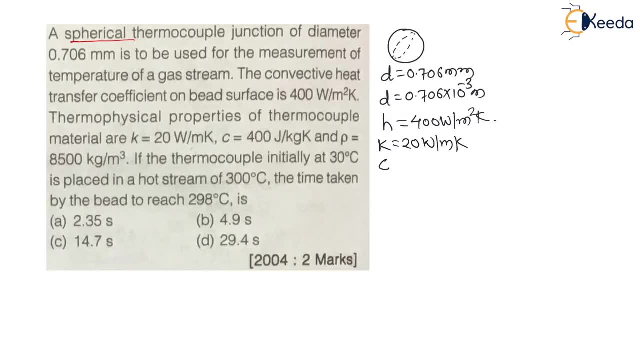 given 20 Watt per meter Kelvin. Specific heat C is given 400 Joule per kg Kelvin. Then density is given 8500 kg per meter cube. Here you will find these values If the thermocouple initially at Now. this thermocouple is initially at 30 degree Celsius, That is initial temperature of solid. 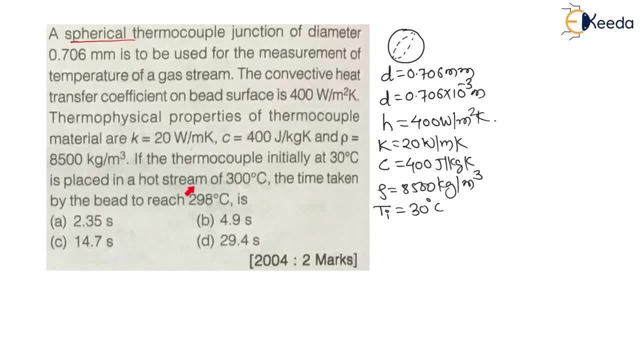 Then it is placed in a hot stream of 300 degree Celsius. Now here stream temperature is given. Therefore it is a fluid temperature. gas stream: It is a gas stream. Therefore it is a fluid temperature. Therefore it is T infinity, which is 300 degree Celsius, The time taken by the bead. 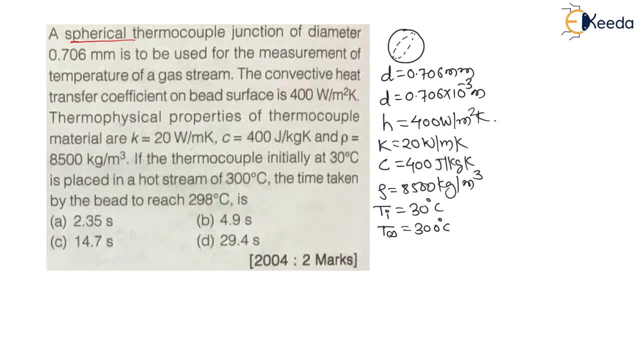 to reach 298 degree Celsius is Now to reach temperature of 298 degree Celsius. what is the time taken by this bead? in second, Because all options are given in second, So let us calculate this time Now. before calculation of this time, let us check whether this problem falls under lumped heat capacity analysis or. 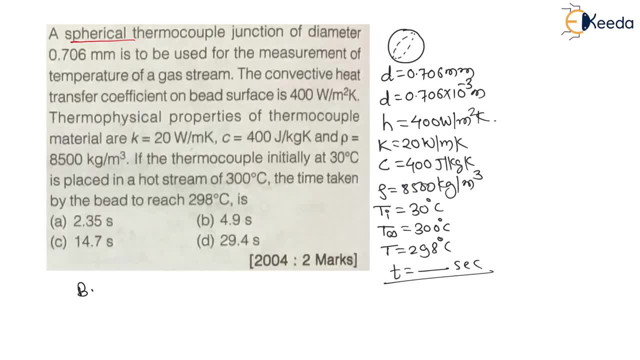 not Now to check that. we have to check Biot number. The Biot number is nothing, but it is H, E, L divided by K. Now, here H is convective heat transfer coefficient, which is given, Here K is thermal conductivity, which is given, And E, L is characteristic dimension. 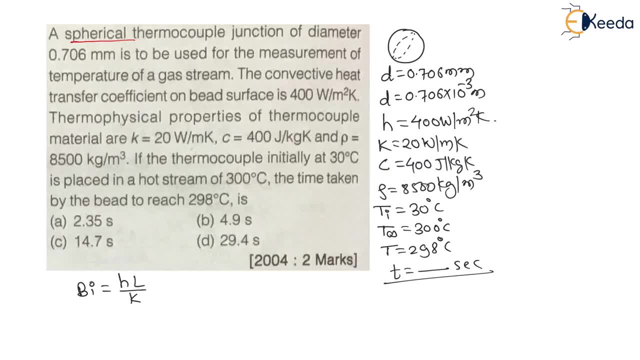 And this E L characteristic dimension, nothing but volume divided by surface area of this sphere. therefore, this l is nothing but volume divided by surface area, which is equal to volume of sphere is 4 by 3 pi r cube, then the surface area of sphere is 4 pi r square. right here, this 4 pi r square will get cancelled and 4 pi r square. 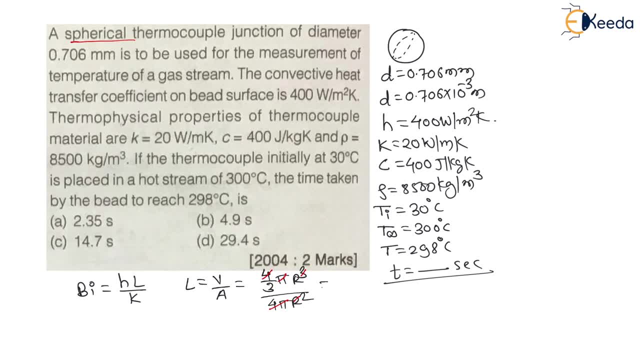 will get cancelled. it will remain r by 3. right, it will remain r by 3 again. can i write? it is diameter divided by 6. r by 3 is nothing, but diameter divided by 6. therefore, it is d by 6. therefore, this is very important, my dear students here, characteristic dimension, which is nothing. 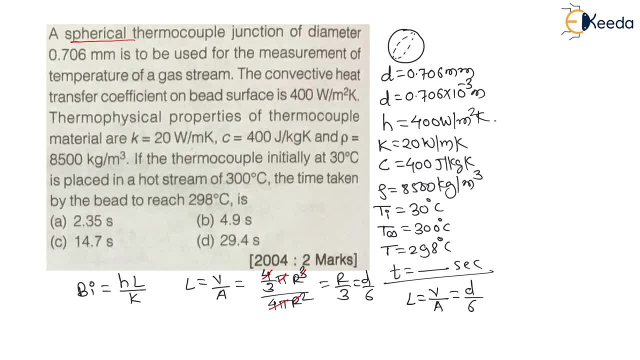 but volume divided by surface area will become diameter divided by 6 for a sphere. right again, therefore, can i say area divided by volume will be 6 by d. latter it is required. this term is required later for the calculation. area divided by volume is 6 by d. now here, biad number is h, l divided by k. 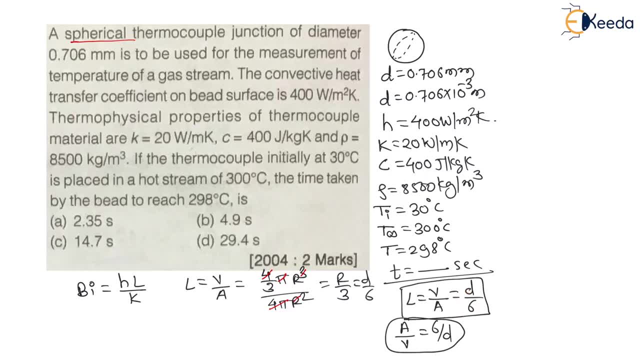 instead of this l, let us put a diameter divided by 6. therefore this biad number becomes h d divided by 6 k. so let us put the values now. h is given 400, diameter is given zero point 7, 0, 6 into 10 to the power minus 3. 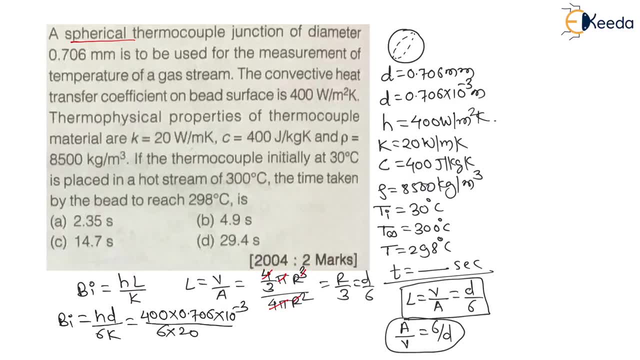 we have a 6 into thermal conductivity, k is given 20, so let us find this answer. so, my dear student, this biad number will be 2.35 into tenth power minus 3, and definitely it is less than 0.1, right? definitely? 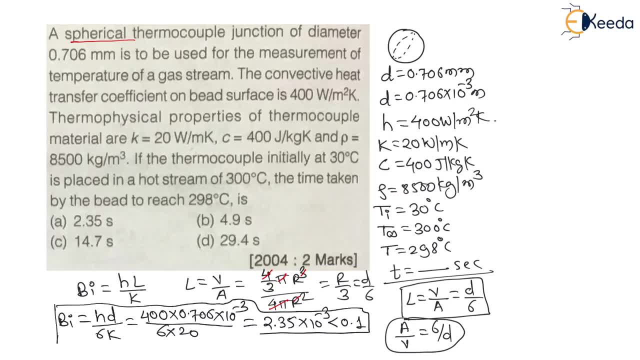 this biot number, calculated by us, is less than 0.1. now, my dear students, we know this biot number is less than 0.1, then the problem is always lumped analysis problem. therefore, here i will say: it is a problem of lumped analysis. lumped analysis, right, so we can use all formulas of lumped analysis. 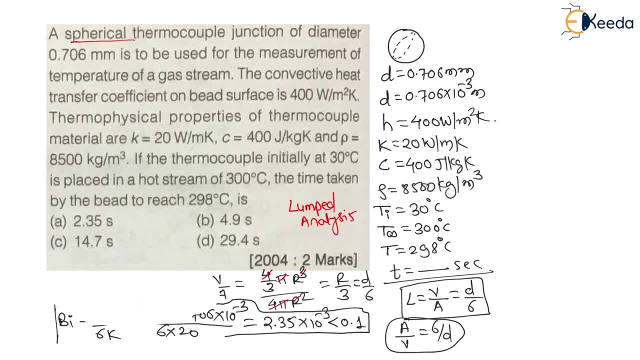 so let us use these formulas and find the required parameter, that is, time is required, so let us find this time by using lumped formulas. now, my dear students here, lumped analysis formula is nothing but temperature t minus t infinity divided by t. i minus t infinity is equal to e, to the power. 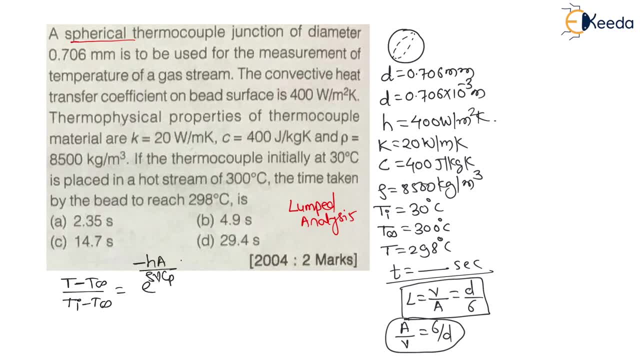 minus h a divided by rho, v, cp into time t. this is called lumped analysis problem formula right, where t is the temperature after time t. t infinity is stream temperature, that is, fluid temperature. t i is initial temperature of this bead right e. h is convective heat transfer coefficient area divided by volume. we have seen: 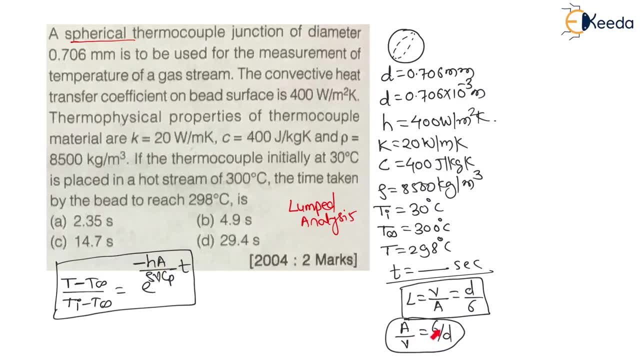 6 divided by d. so, instead of this area divided by volume, we will replace by 6 divided by d. now, rho is density, t, p is specific heat and t is the time right. so, my dear students, let us use this formula here. i am going to erase this question so that we will get sufficient space for the solution. 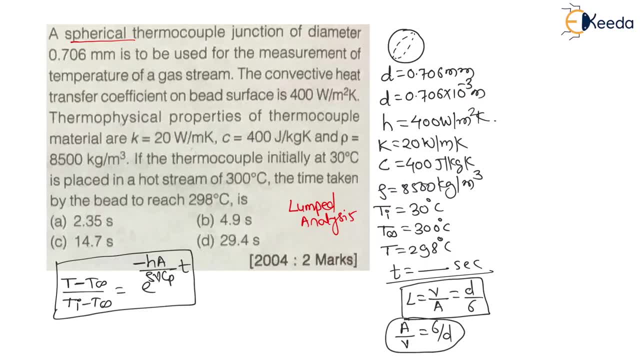 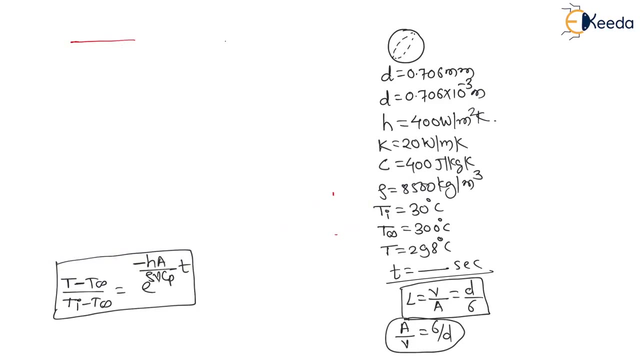 now here only i will tell you answer, my dear students. answer is: let us pause this video and find the answer. the answer will be option b, that is, 4.9 seconds. right, let us check how this answer will come right here. i am going to delete the question. so, my dear students, as lumped analysis formula is valid, so let us use this. 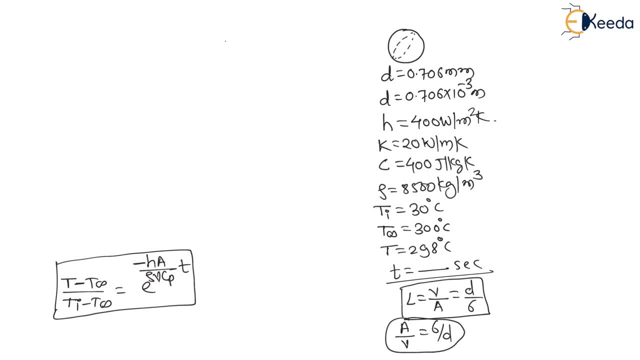 formula. therefore: here, area divided by volume, we are going to replace with 6 divided by d. therefore the formula becomes: t minus t infinity divided by t. i minus t infinity is equal to e, to the power minus h into t. you have a rho. tp into area divided by volume is 6 by d, 6 by d, right, so let us put the values. t is given 298. 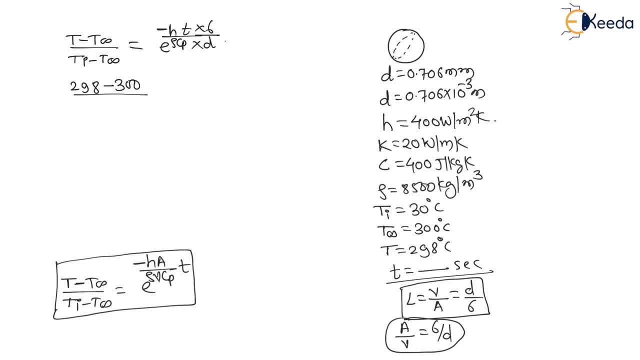 right. t infinity is 300. you have a. ti is 30 minus 300 is equal to e. to the power, h is nothing but 400 minus 400. into time. we have to calculate into 6. you have a density is given 8500, 8500 into. 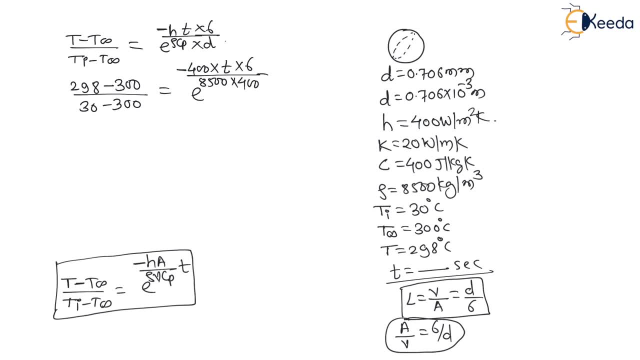 is given, cp is nothing but 400 into diameter. d diameter is 0.706 into 10 to the power minus 3. into 10 to the power minus 3. all right now, my dear students, let us simplify this equation again. therefore, here, equation will be: minus 2 divided by minus 270 is equal to e to the power. here this: